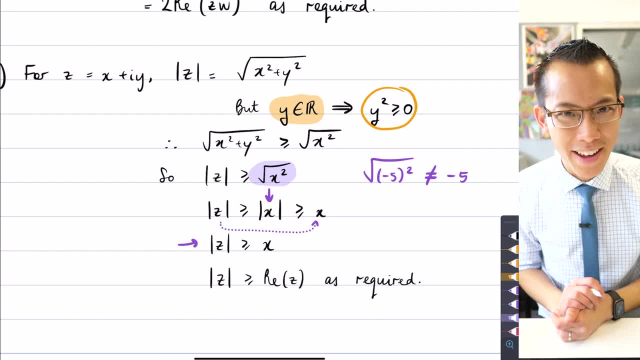 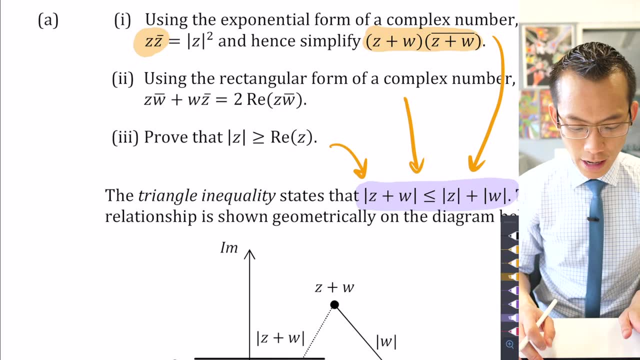 So that was part three. At last, we have laid all the foundations. What was the point of proving all these results? We're going to use all three of them when we do this. proof of coming back to the question: the triangle inequality. Remember all three of these pieces: one, two and then three. 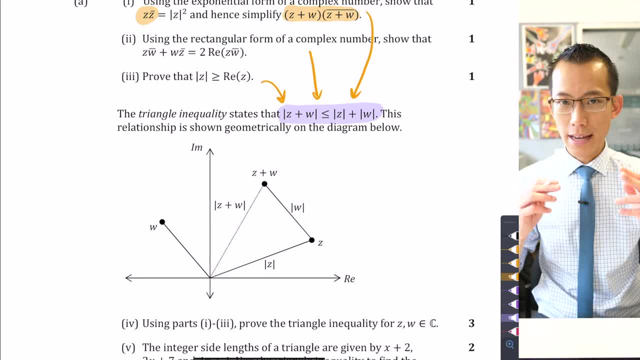 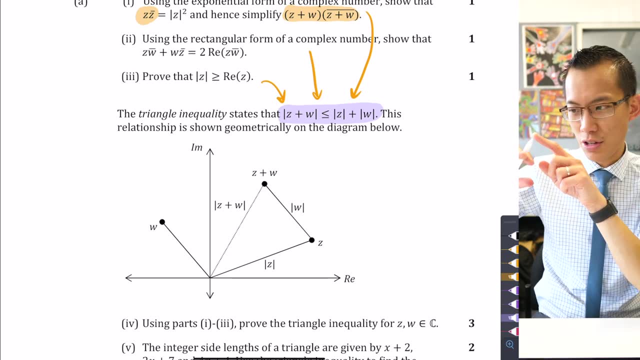 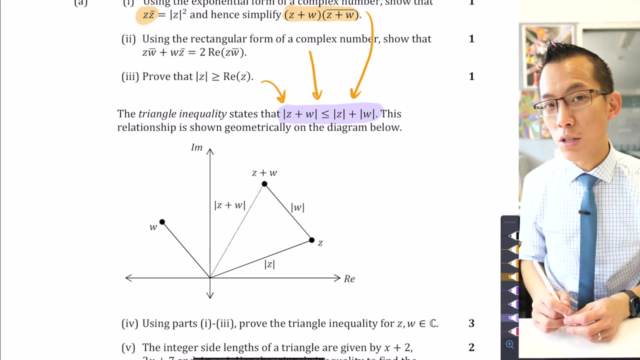 they're going to feed into here. Now, I'll admit, this is quite tough. You're more used to seeing part A and then, hence, part B, And so you only have to keep one thing in your mind that you're going to use for the next bit. But here, because you've got three parts to use, that makes it much. 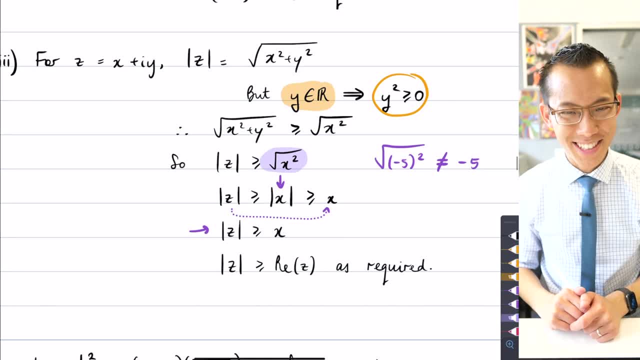 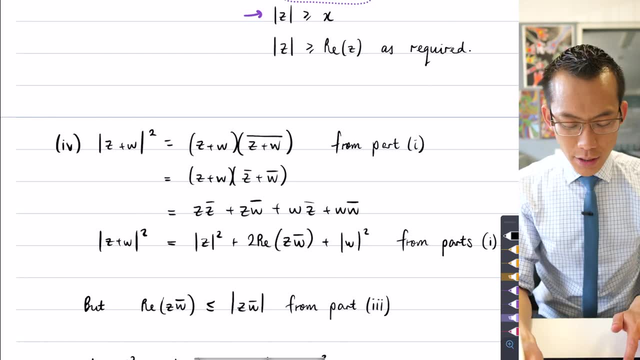 more challenging, And that's part of what we signed up for in extension two. So let's have a go at part four. I didn't even write part four. Let's do that, Okay. So the first thing I'm going to say, 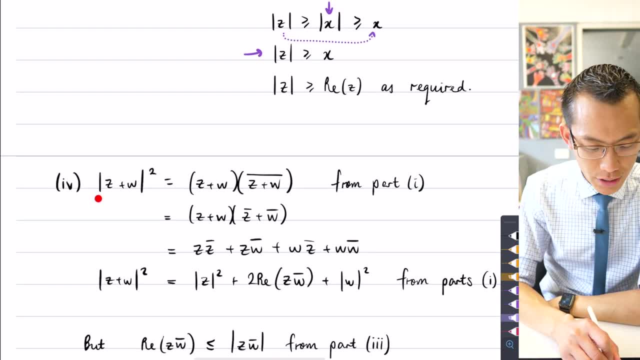 is. I'm dealing with the modulus of Z plus one. all squared, I can say that it's equal to Z plus one times Z plus one bar, And that was literally where I finished part one. Okay, Now, the reason why this is a helpful thing to say is because it gives me the modulus of Z plus one. 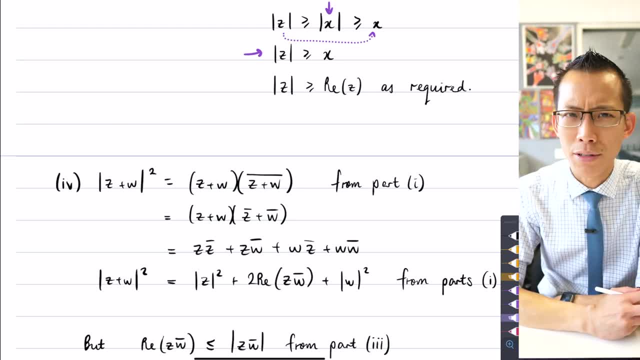 all squared And I need the modulus of, not Z plus one, Z plus W. I need the modulus of Z plus W because it appears in the triangle inequality. So this is like a stepping stone to be able to work with the modulus of Z plus W. I at least know something with the modulus of Z plus W squared. 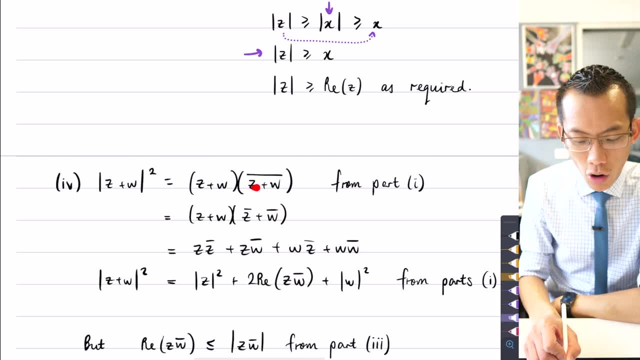 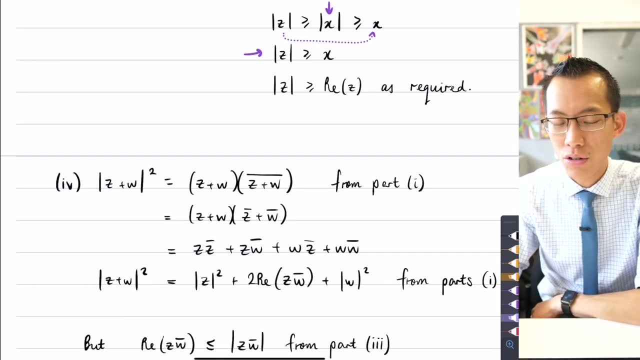 So I do that. You can see here, the conjugate of a sum is the sum of the conjugates. You can just plug in the conjugate of a sum. You can see here that the conjugate of a sum is the sum of the. 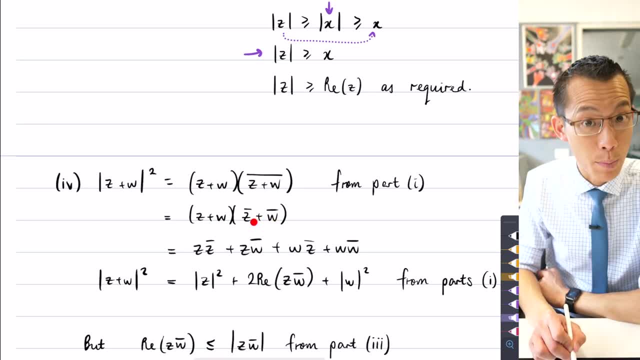 conjugates. That's one of the properties of complex numbers and their conjugates that we saw in the syllabus and we've proved a while ago. So I'm going to put that down there as a very minor simplification, And once I've got that, I'm just doing a binomial sort of expansion here, right? 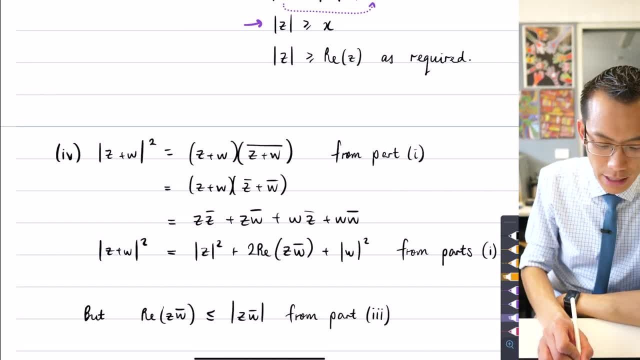 Binomial here, binomial here, And I'm just going to multiply all these terms together Now. I hope when you just did the expansion, you then noticed: wait a second, this looks very familiar. This is Z W bar plus W Z bar, which we have actually. 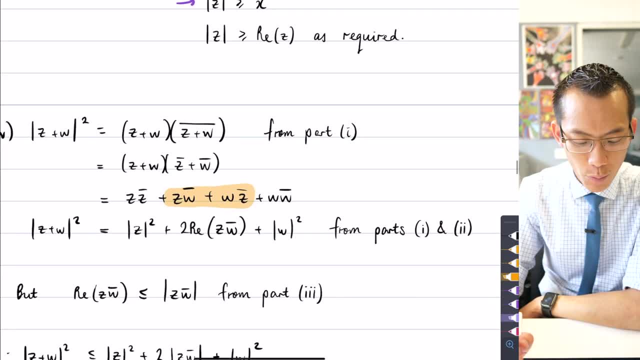 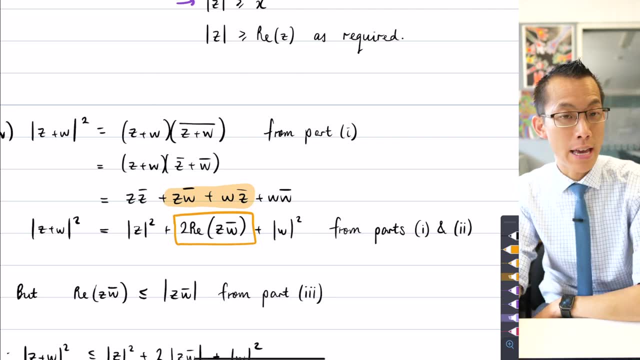 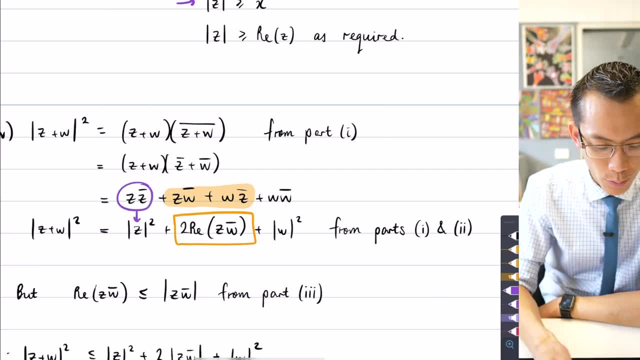 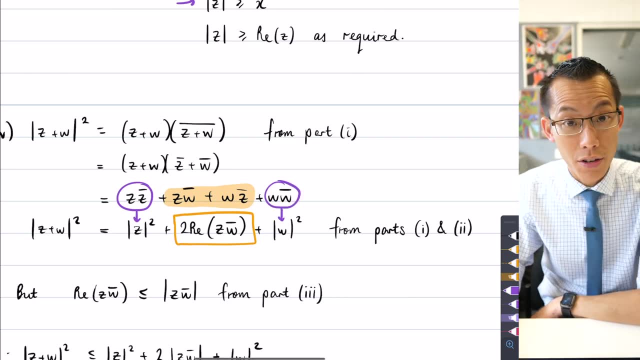 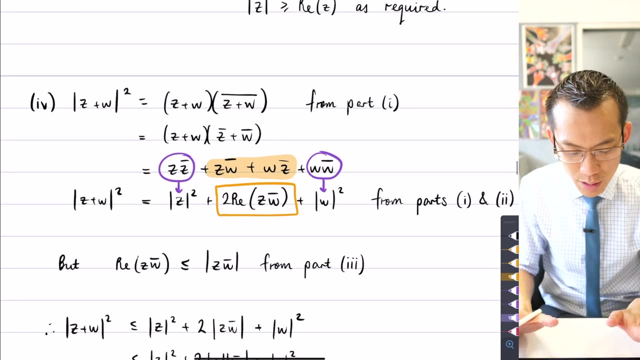 we saw z z bar. that was the square of mod z and by the exactly the same logic, w w bar is the square of mod w. so I've done a bunch of substitutions here off the basis of part one and part two. so this is good, but how do I work from this to my actual triangle- inequality? well, there's one last. 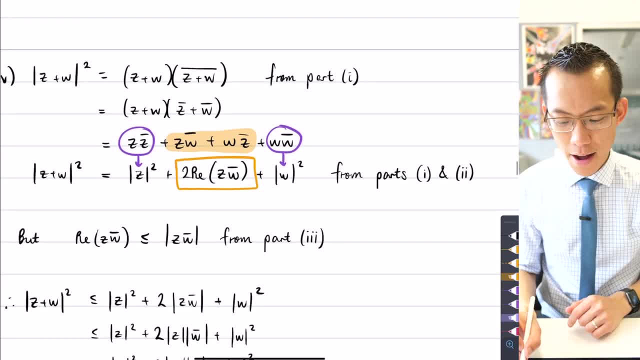 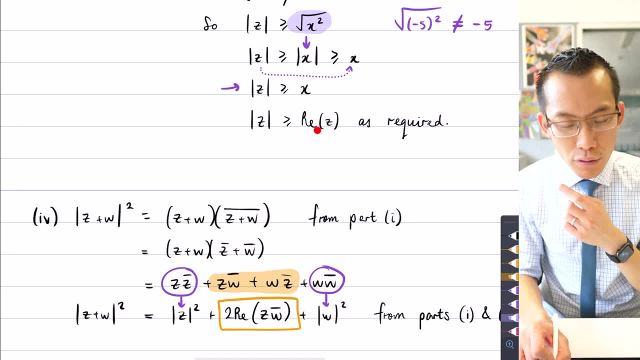 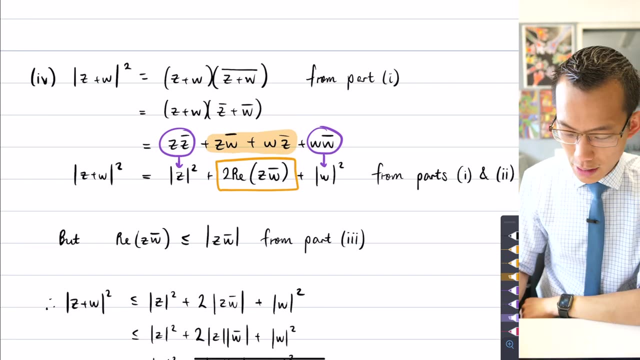 part I haven't used yet and that is the part three, the one I just most recently did, which had to do with the modulus of the number and the real component of that same complex number. so you can see, in here I can say: hold on a second I've got. 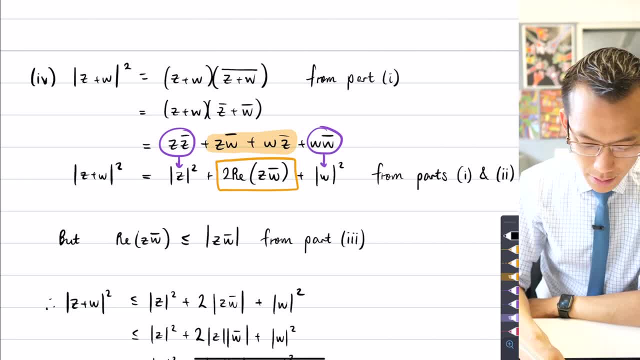 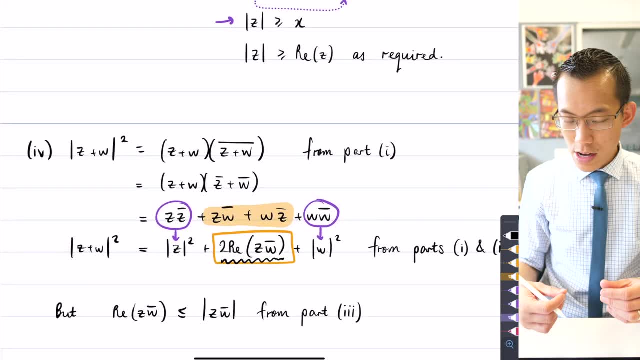 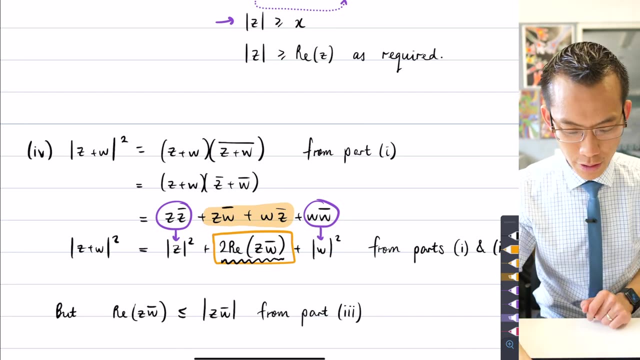 a real component, a real component in here of a complex number, right, and it is lesser than or equal to the modulus of that same complex number. that's what this means here. I've got it written backwards so maybe it would be more helpful if I wrote it in reverse order. I guess the real 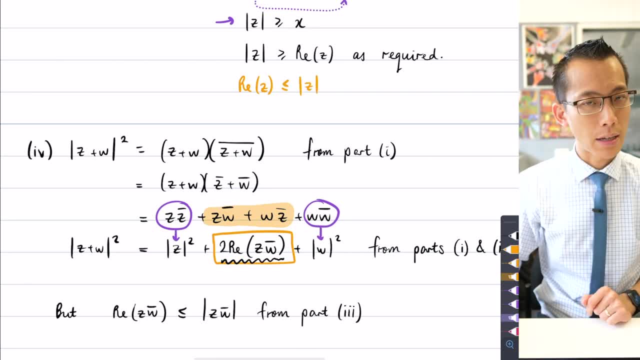 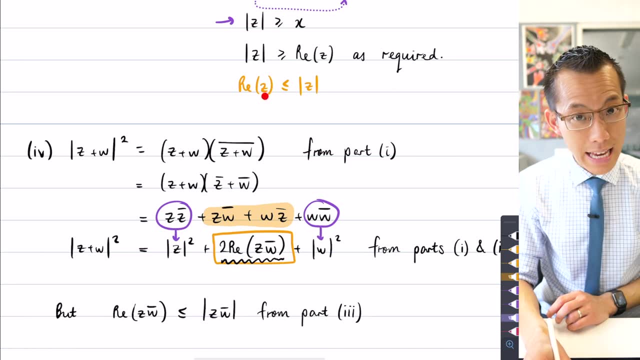 component of z is lesser than or equal to mod z. okay, so I've just switched sides. so that means I've reversed the direction of inequality and you can see that I've got a real component of z. so my solution here is to substitute the integral I live for, which is actually a rather 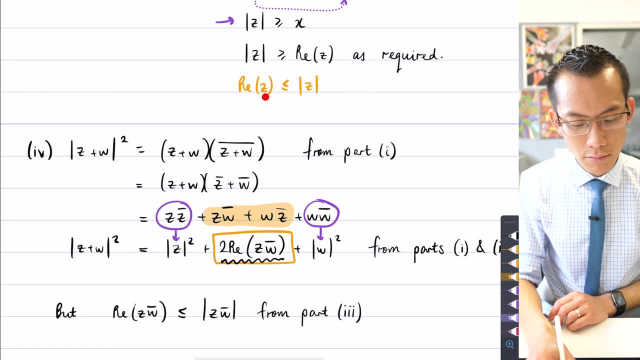 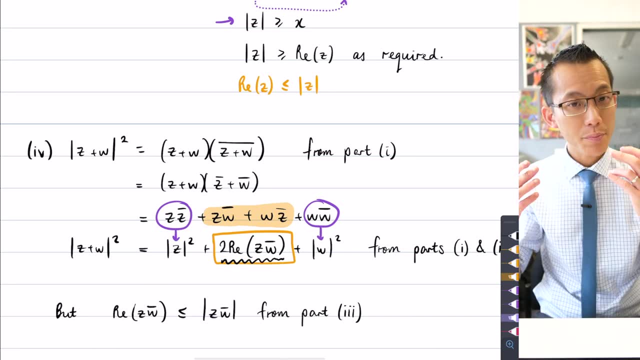 less than or equal to mod z. if that was yes these days, if I would substitute episodes, yo, if I were to substitute instead of writing z, if I were to write z w bar, then I could put: the real part of z w bar is less than or equal to the modulus. what a z w bar. and that is indeed exactly what. 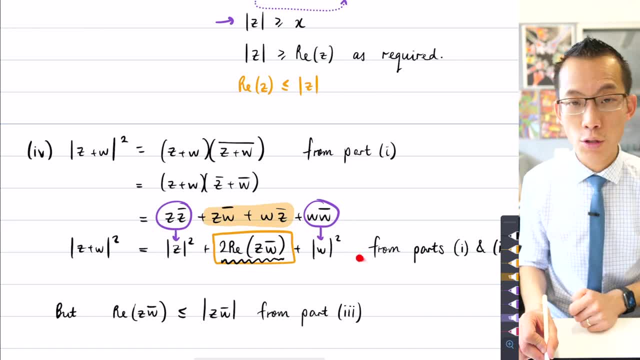 I've written here. that was what I had from part 3, and the reason why this is so powerful is because then I can turn this equation, which has lots of true stuff but isn't what I'm trying to prove, because I need the triangle, Ina. 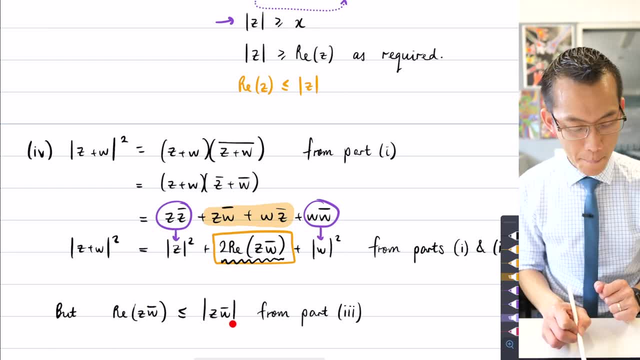 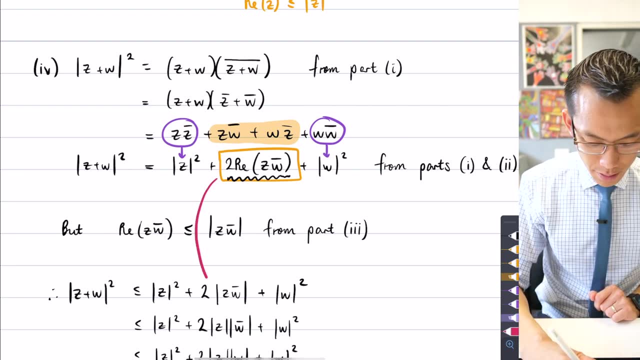 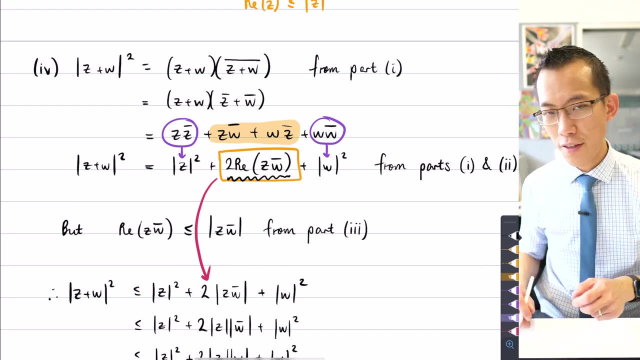 Yeah, substituting something smaller for something bigger, right? So you can see here because I have substituted- let's make the connection in here- I've substituted this for something bigger than itself. So now the right-hand side, instead of doing you know, we're used to thinking of. 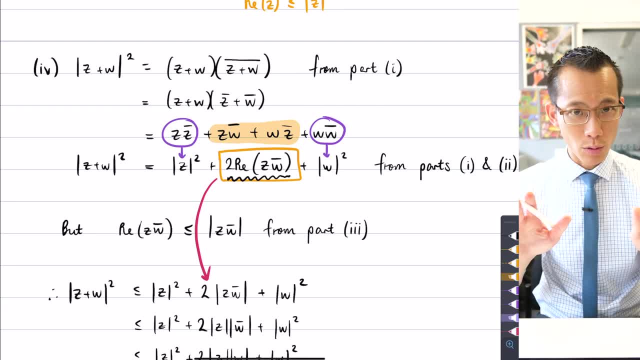 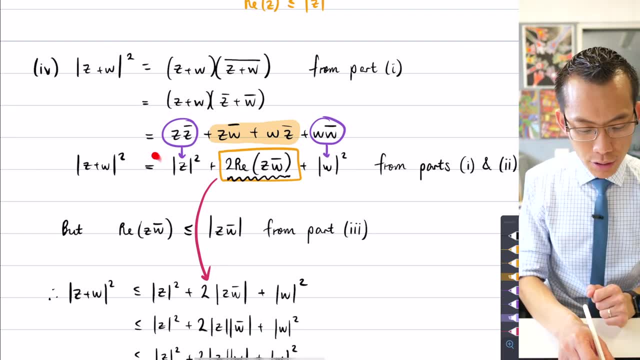 substitution, as do something for something which is exactly equal, but I've now put in something in its place that's bigger, heavier, right, It's greater in value. So now, instead of the two sides being equal, well, the side where I put in something bigger, something larger, it's now. 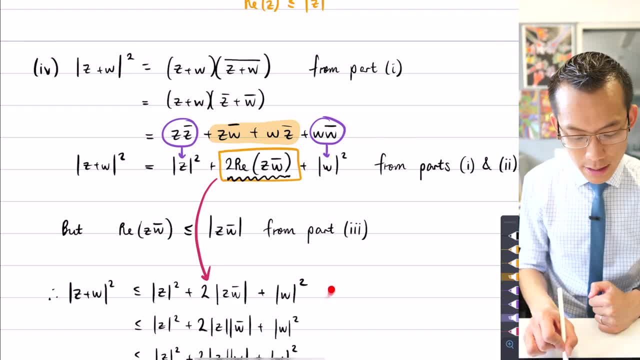 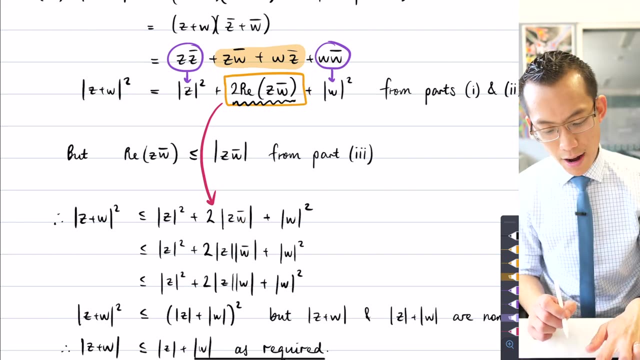 bigger than the other side. Do you see that? So the right-hand side is now bigger than the left-hand side. In other words, the modulus of z plus w, all squared, is smaller than all of this stuff over here. So, going from here to the next line, you can see I've again. 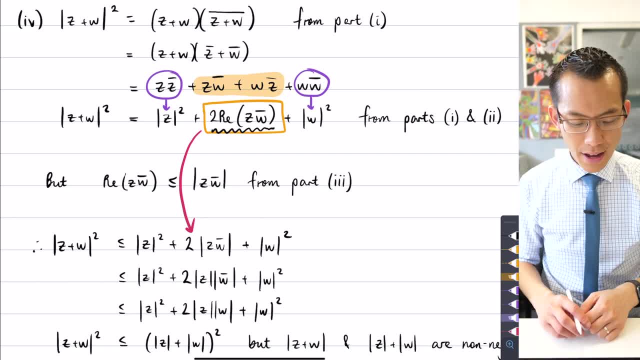 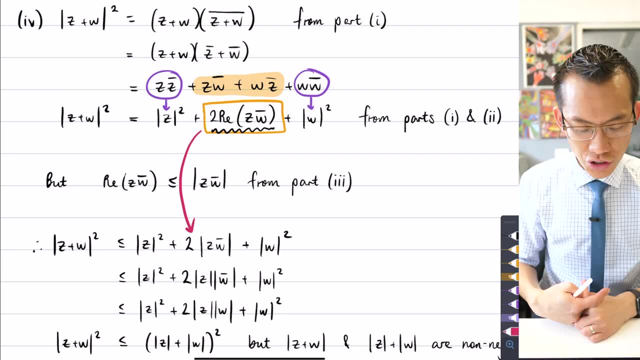 used the same thing over and over again, So I've substituted this for something bigger, this result that I've seen earlier, which is that the modulus of a product is equal to the product of the moduli. I actually proved that in a much earlier question. to do that graph with the 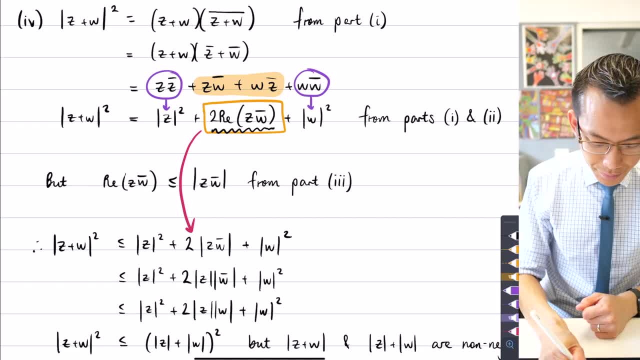 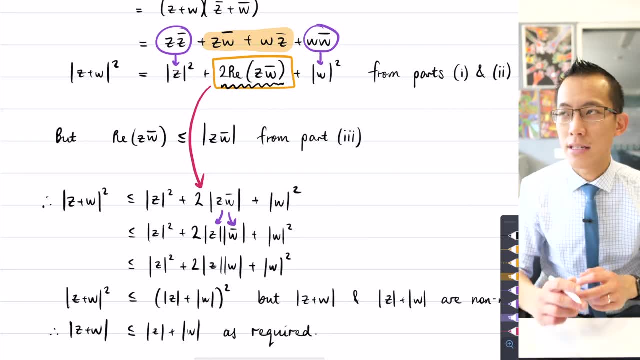 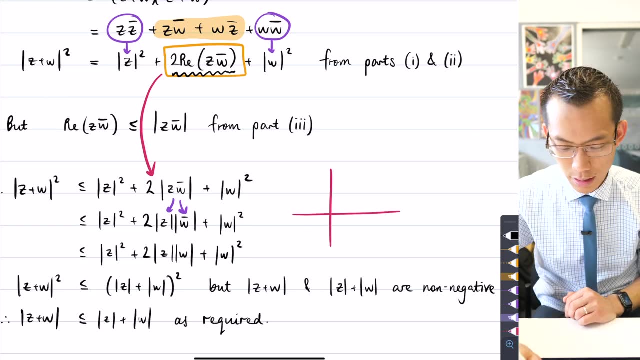 two hyperbolas next to each other. So I've split this apart into its two components. And the thing about the modulus of, say, a conjugate is that what you've done is you've reflected to the opposite side of the real axis. So, for example, if I were to place, let's place, w, 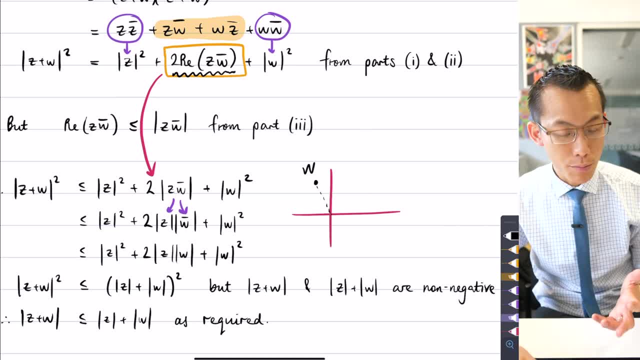 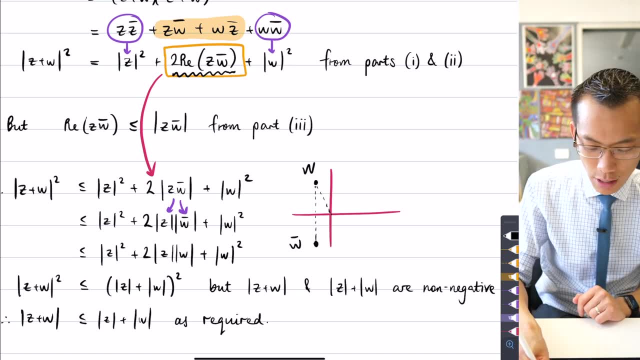 say over here, suppose that was w, where would w bar be? It would be reflected across the real axis And so, if you have a look, this is going to be the modulus of w bar, this is the modulus of w. 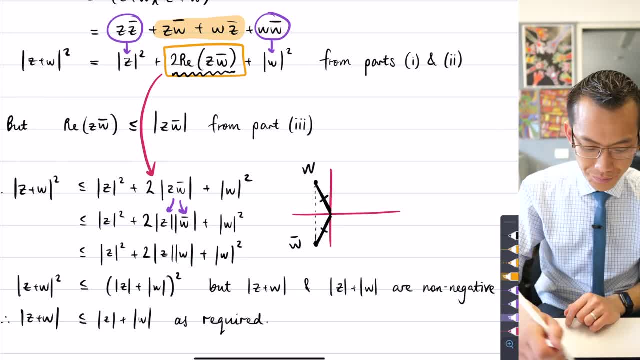 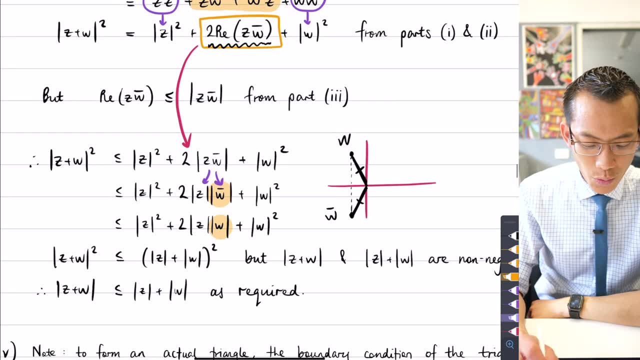 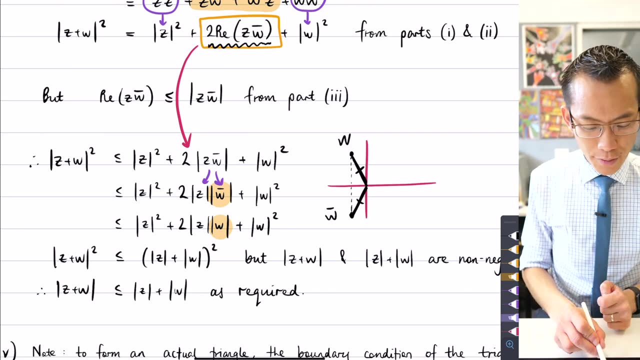 and you can see that these two lengths are equal. So what I've done is I've substituted that modulus of w bar with just the modulus of w. okay, And what I've done here beautifully is I've created a perfect square. Do you see that This is in the form a squared plus 2ab plus b squared. 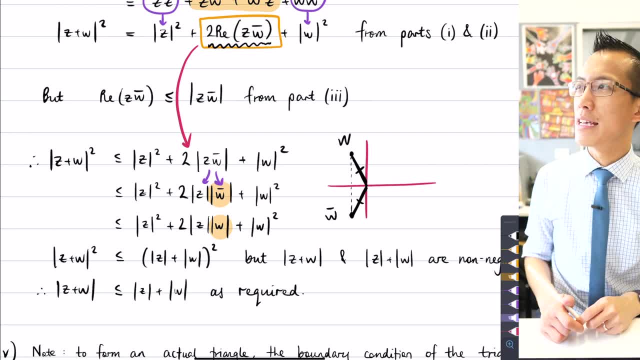 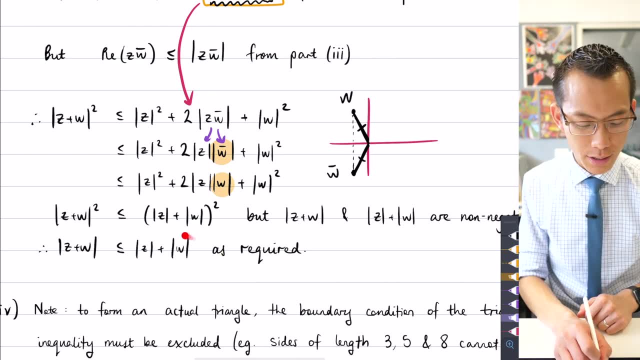 Perfect square. it's just that the a's and the b's happen to be the moduli of complex numbers. So this here is the a plus b, all squared, but instead of a and b I've got mod z and mod w. okay, 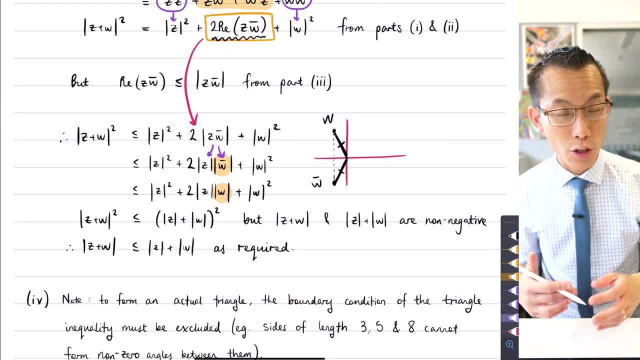 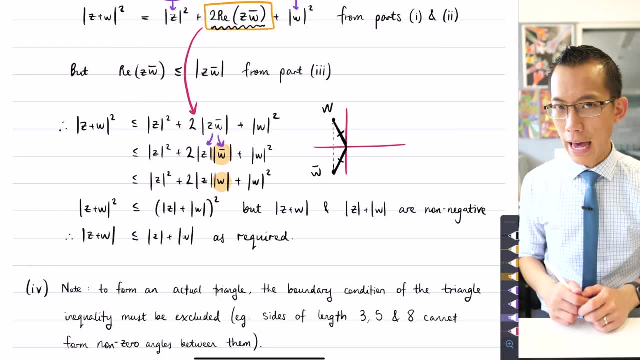 Now we're so close. I mean you can see my final line already here. It is the triangle inequality. But a major thing that lots of people forgot to take note of is that the triangle inequality is the fact that you cannot simply have a squared is less than or equal to b squared and then say: 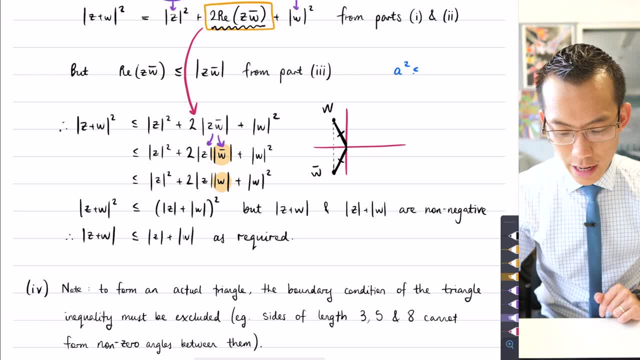 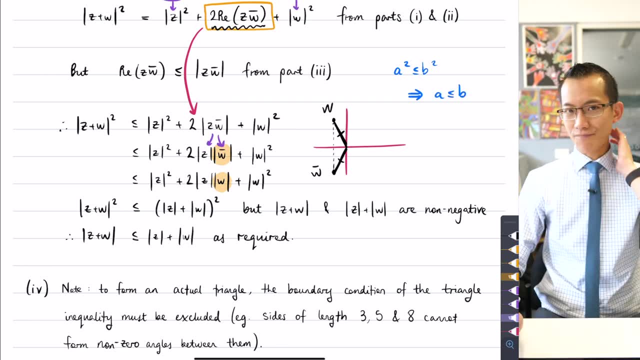 in fact I should write that down. you can't say that a squared is less than or equal to b squared and think that that implies that a is less than or equal to b. This is not always the case and it's fairly easy to think of a counter example If, for instance, I said: 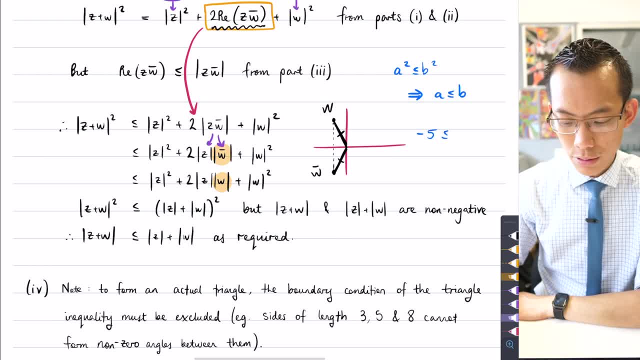 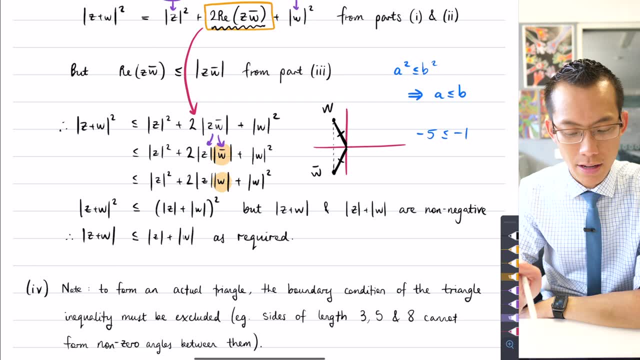 hmm, negative 5 is less than or equal to negative 1, that's a true statement, isn't it? You've got something much more negative over here, so that's why we say it's lesser than Can I say. therefore, from negative 5, all squared. 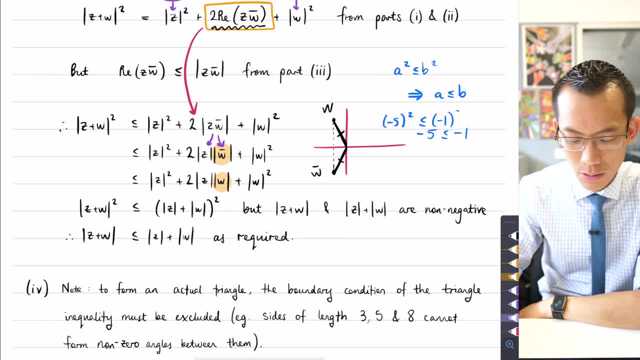 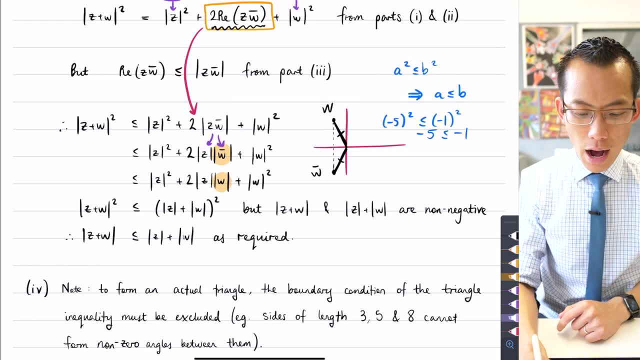 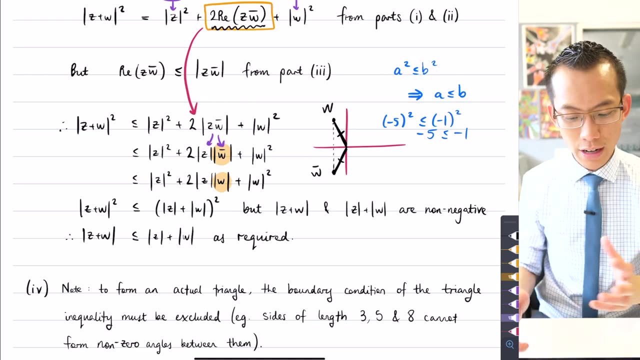 is less than negative 1 all squared, do those two things follow? Is there a logical connection between them? And you can see this is plainly untrue. So I can actually say no. hold on a second. something is going wrong here. I can think of other examples where you know I've got an. 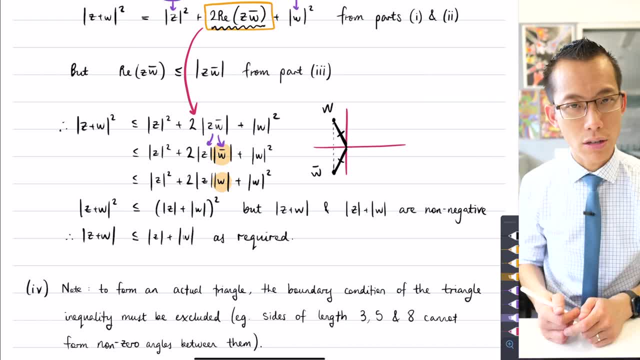 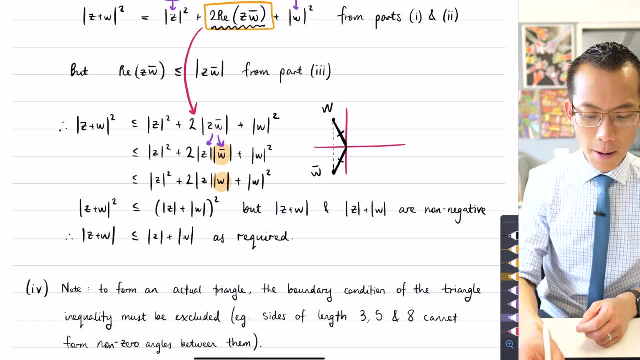 set of inequalities that flows one piece to the next. The real issue here is negativeness. When you've got negative numbers flying around in inequalities, they really mess things up right. So therefore, the real issue or the real solution for this is to say: but the things on both sides 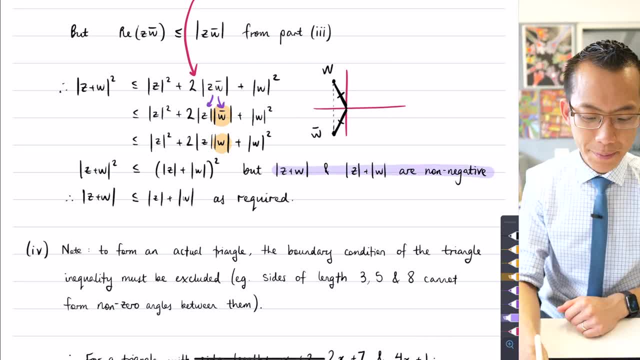 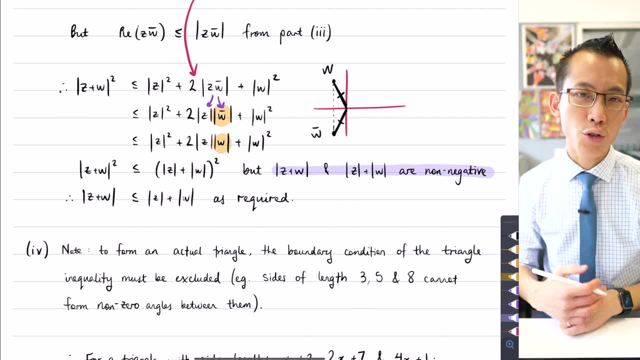 they're magnitudes, So therefore they are non-negative, right. So since they are non-negative, I actually can take the square roots of both sides and I get a valid result, In other words, the triangle inequality. So that was done quite poorly. Very few people. 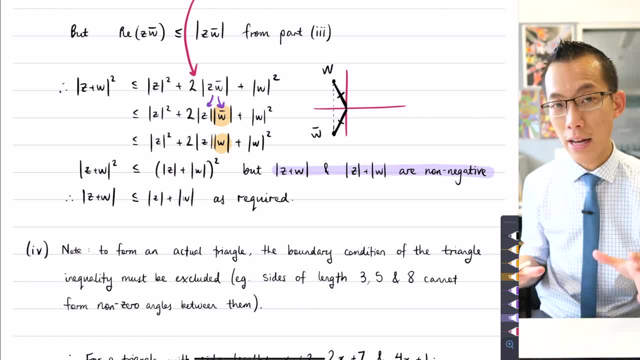 made a statement about the fact that you've got both sides being positive. So therefore, if their squares are in a certain size order, size relationship, the same thing is true of the original numbers. So that's what I've done, from this line to this line. Okay, so I'm so very. 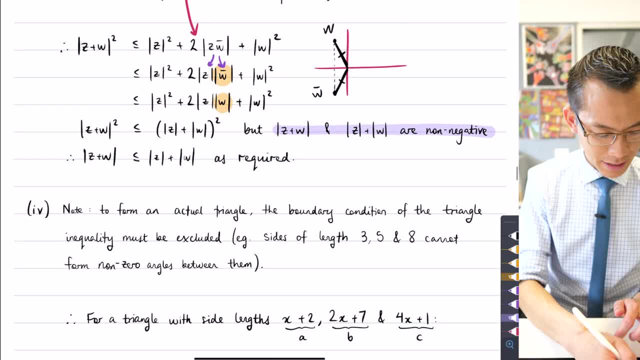 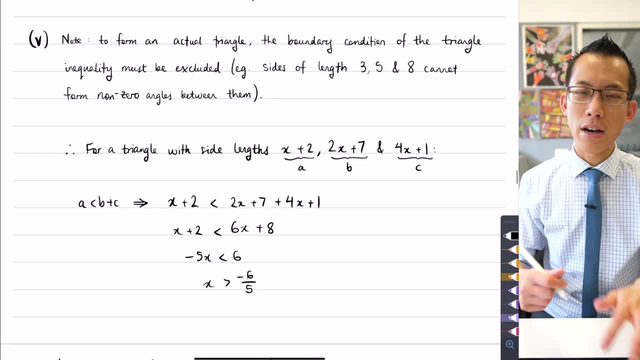 close, I think. yeah, I made a mistake calling that down here. part four, It's actually part five, So let's fix that up. I've done part four. Now in part five, what I have to do is use the triangle. 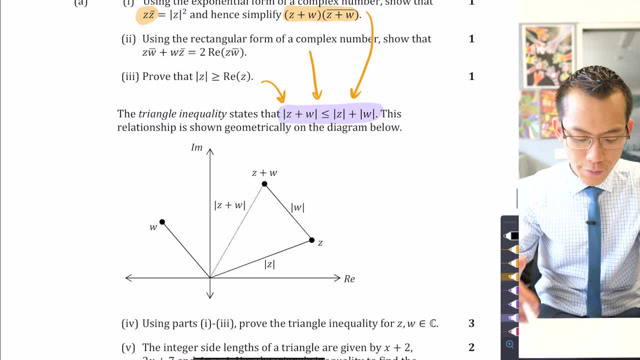 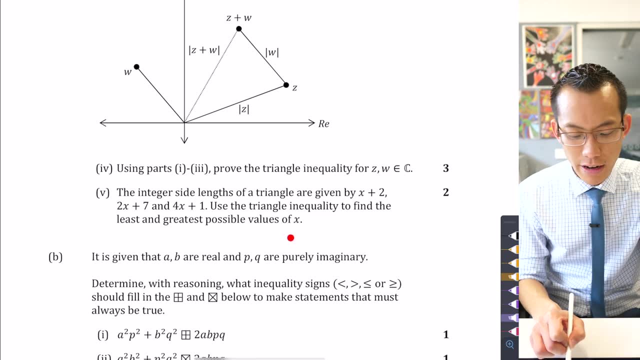 inequality. to actually find out, let's have a look. If I've got a triangle- and I know its sides, are these lengths: x plus two, two x plus seven and four x plus one. what are the least and greatest possible values of x? Now we have to do better than just to sub in values, right? The question? 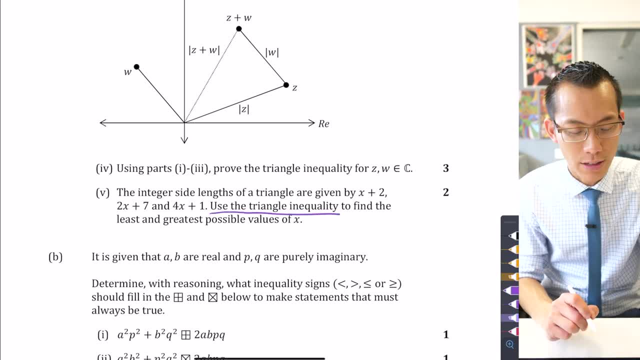 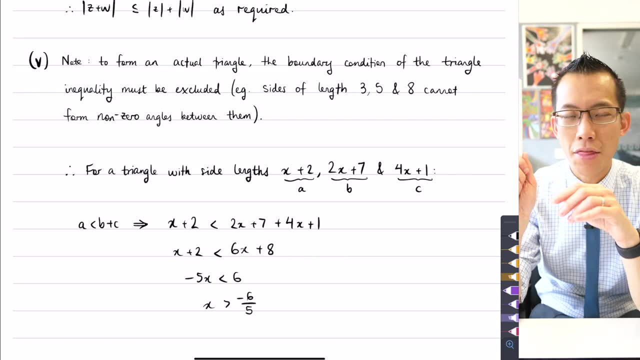 itself specifies: use the triangle inequality. So how do I do that? Well, remembering that the whole idea is that in the triangle inequality, it's telling you that you can't have a third side of a triangle that is longer than the sum. 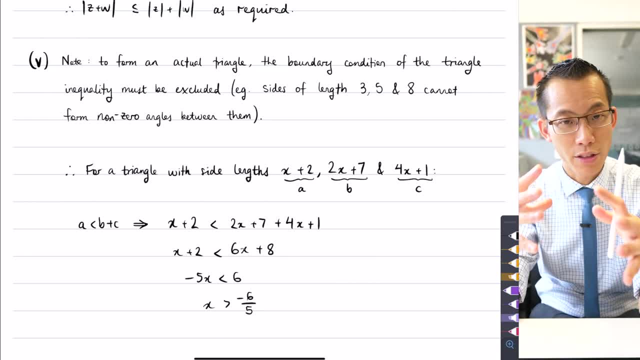 Of the other two shorter sides. right? That's impossible because the lengths would not, the sides would not connect to each other. right Now, this is true for every like. when you don't know which is the longest side, you have to be able to say that it's true for all of them. right? I can say: 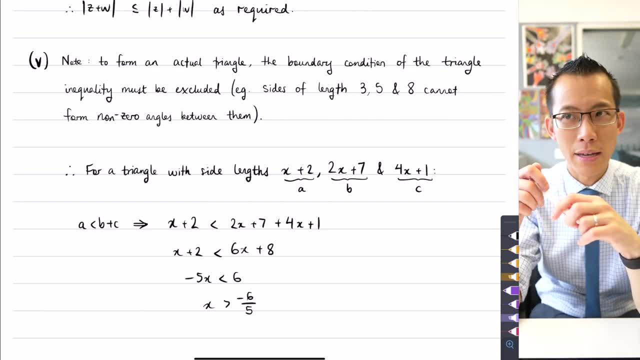 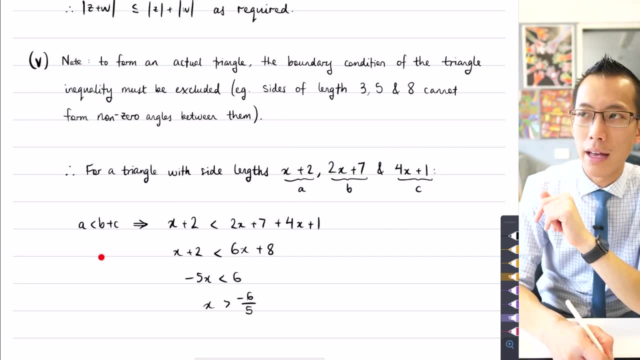 that if the sides are A, B and C, that A is going to be less than B plus C, And that's what you can see. I've written here. But you can also say that of B it's got to be less than A plus C and C has. 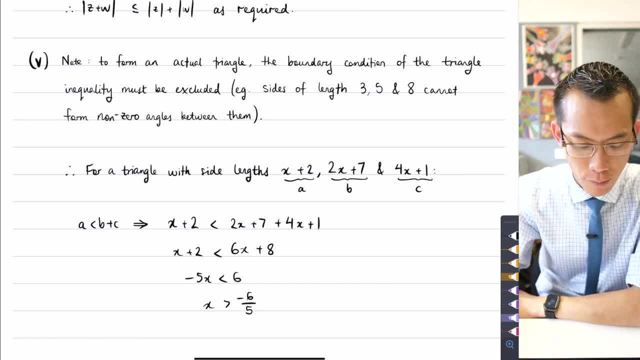 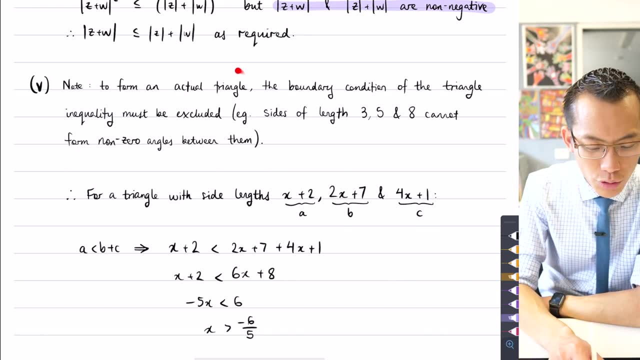 to be less than A plus B. The triangle inequality is symmetrical. It works all the way around. So I'm going to start writing these inequalities, But before I do that, I want to make this note here: to form an actual triangle, right, We actually have to exclude the boundary condition of the 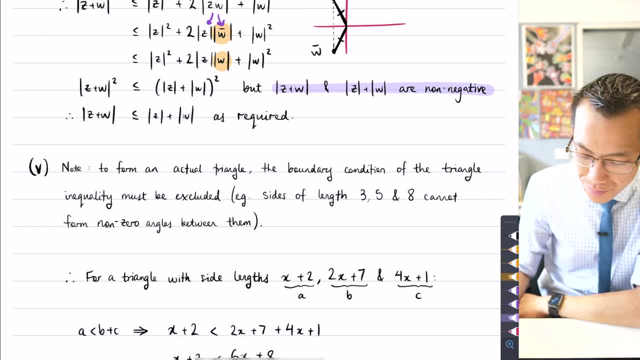 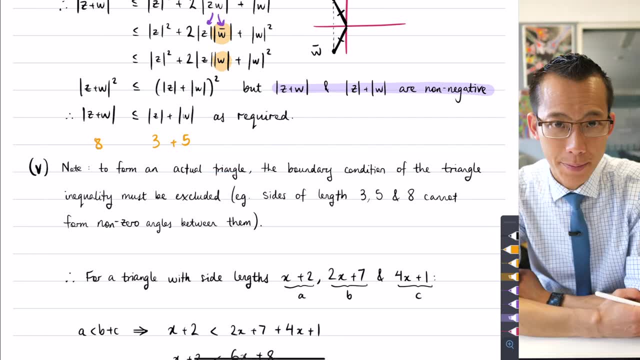 triangle inequality. Here's the triangle inequality here. And if I gave you that example before of one side being three and the other side being five, could that other side be eight? And the short answer is: in theory it could be, But practically speaking, to get an actual triangle out of the 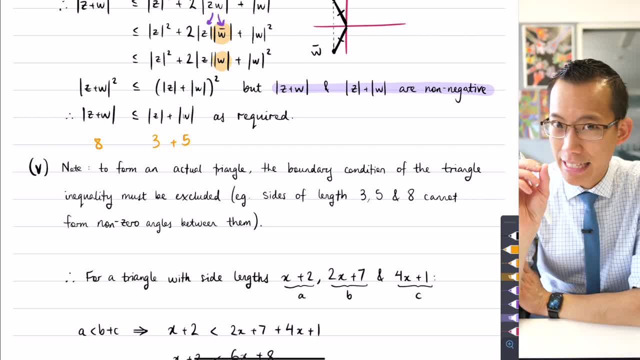 triangle- inequality- I have to say, well, B plus C is less than B plus C. So I'm going to write this down And I'm going to say: well, it can't exactly be equal to eight, because then you've got just a. 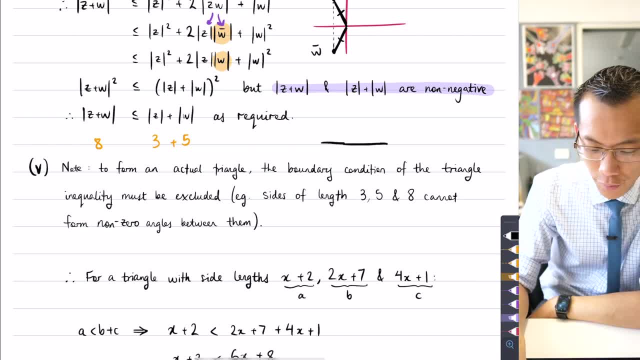 flat geometric object. You've got a three, and then you've got a five, and then the eight just sits right over the top And there's no area to this thing. So it's not actually a triangle. So that's why here I say the boundary condition must be excluded, So instead of saying it's less than 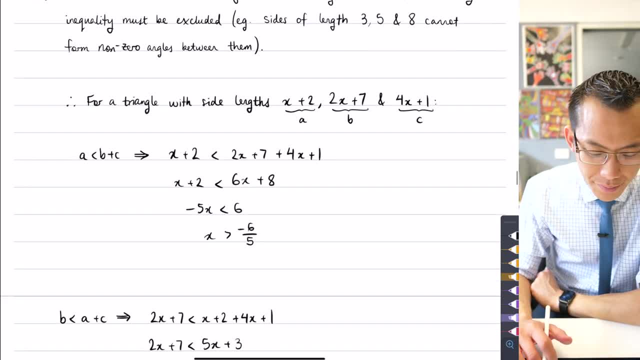 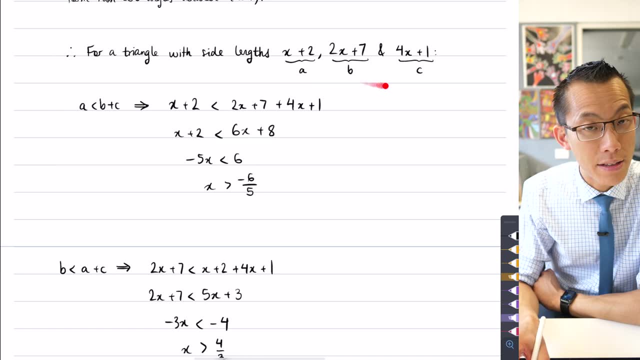 or equal to. I'm going to say it's just lesser than Now. I then have to start thinking about: well, let's have a look at each of the sides and how they relate. So here is me saying: let's call them A, B and C. 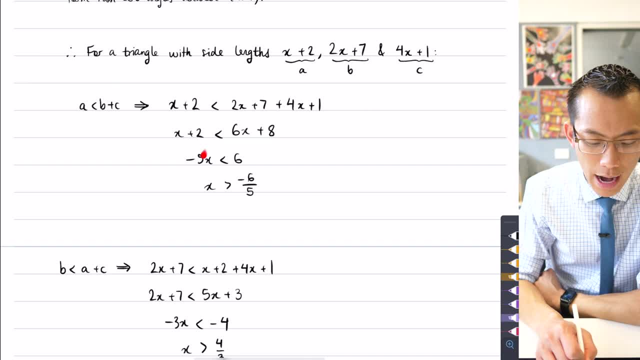 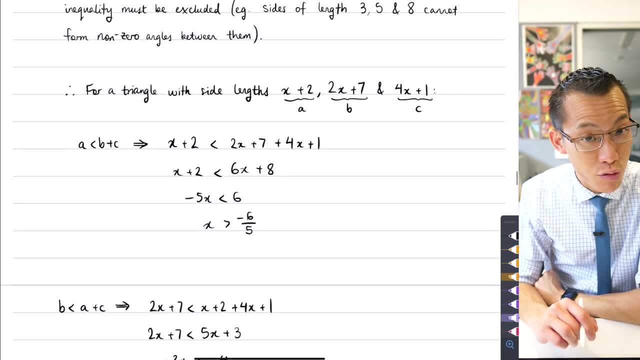 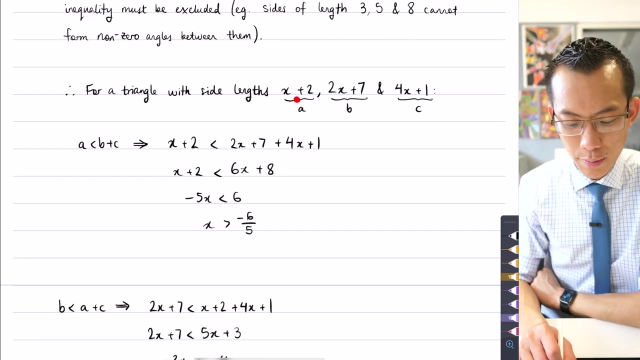 So I can put that in and then just work out the inequality and say this: right? So I'm like X is greater than negative. six on five. Well, that's true, but I sort of already knew that, because you can see this side, here is X plus two, So you know it's going to have to be bigger than. 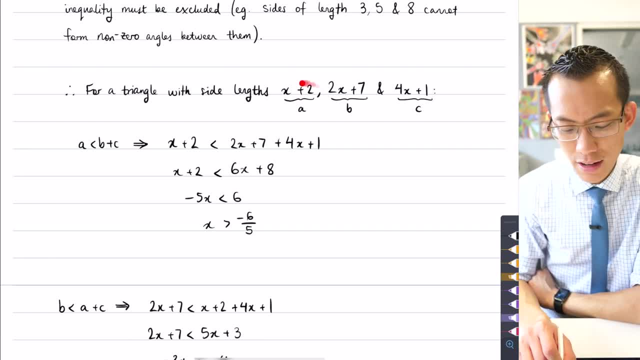 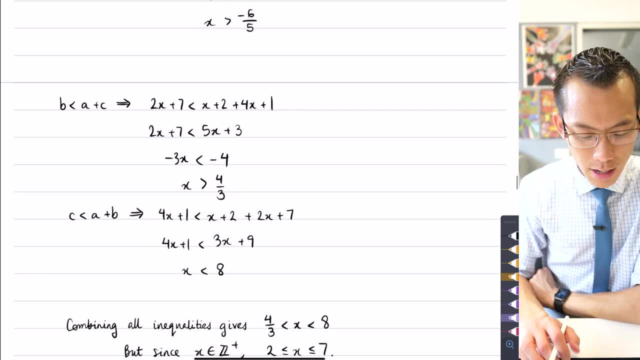 negative two. If I had an X of negative two, then this side length would be zero. So I already knew that. So this is telling me something that was kind of already established. But then when I have a look at the other sides, you can see here you get more interesting results when you compare the. 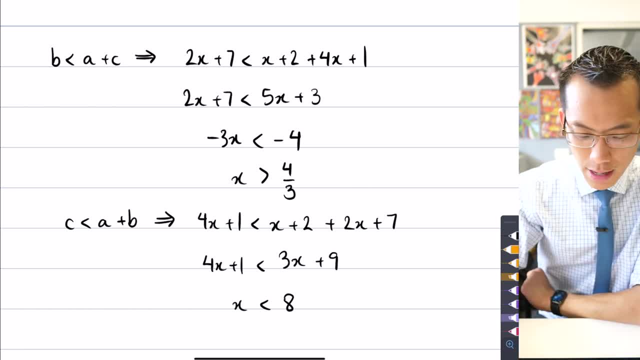 different sides. So here's B and then here is A and C. So when I go ahead and do the algebra for this, I can see that X has to be greater than four thirds. And then, when I do a similar thing down here, here's A again and then here is B. You can see here when I go ahead and do this. 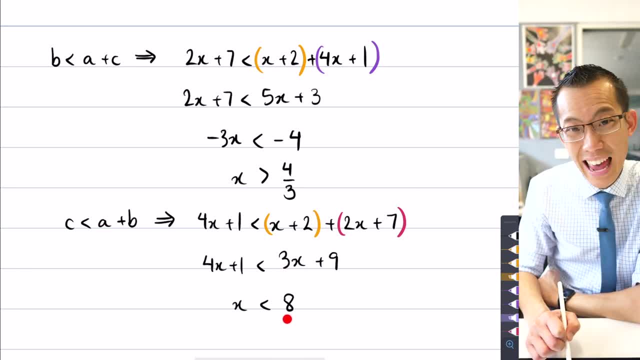 I actually have the inequality facing the other direction that X has to be less than two. Now it's very tempting to then say, okay, well, I've got one inequality here which is a greater than I've got another inequality here which is lesser than So. I'm just between these. 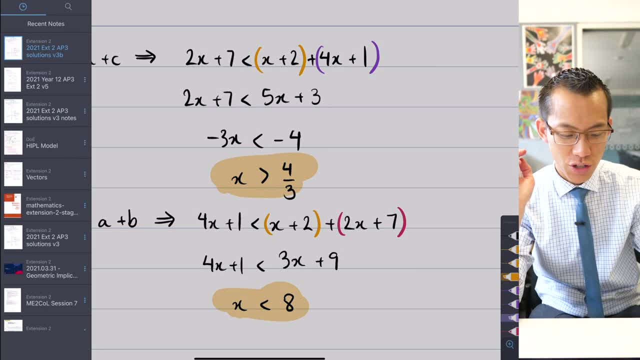 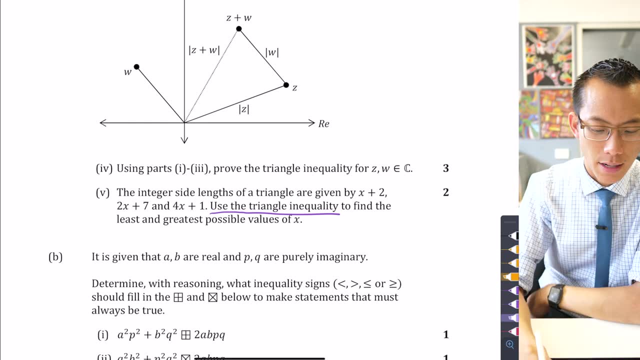 two values. I'm done right, Except if you go back to the question, there's some important phrasing which actually adjusts what we're going to or you know, sort of tempers, the way we're going to interpret this answer, Because you can see here it says that you know you've got the lengths of a 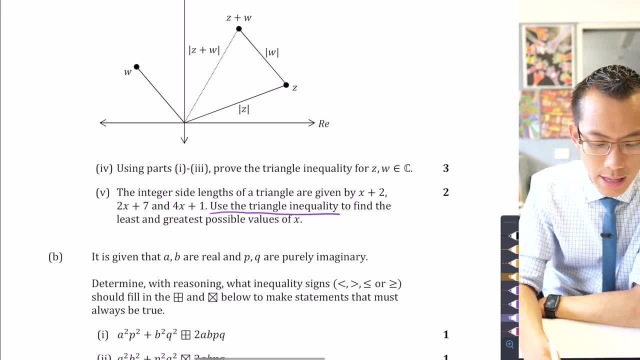 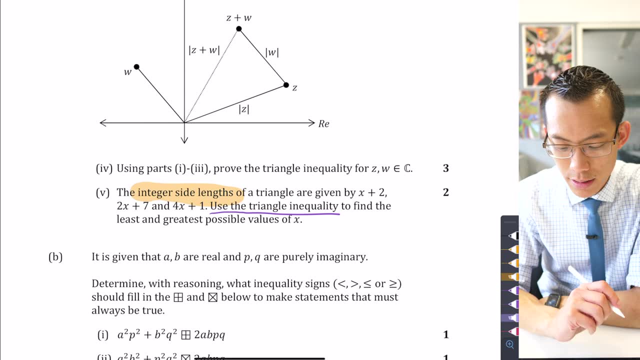 triangle, That's great: X plus two and so on. But it's not just any lengths. These are integer side lengths. That means that the side lengths have to be whole numbers. Now, if the side lengths are whole numbers, that means that, say, for example, this side here, which is X plus two, X has to be. 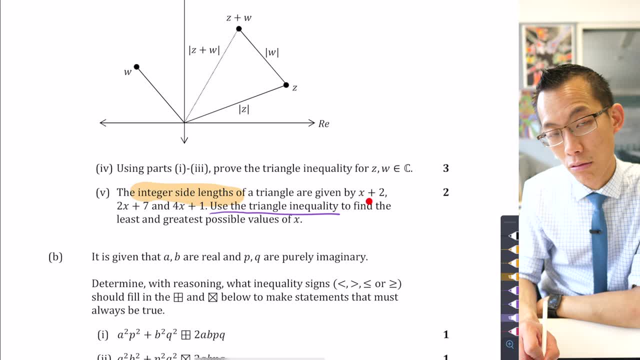 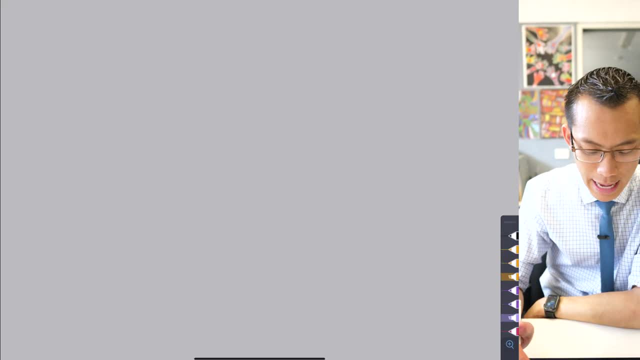 a whole number as well, Because if you have a whole number, anything that's not a whole number plus two, then that won't be a whole number. So X has to be a whole number itself. So what that means is that eight itself. you know I already excluded it because I had to be less than that. 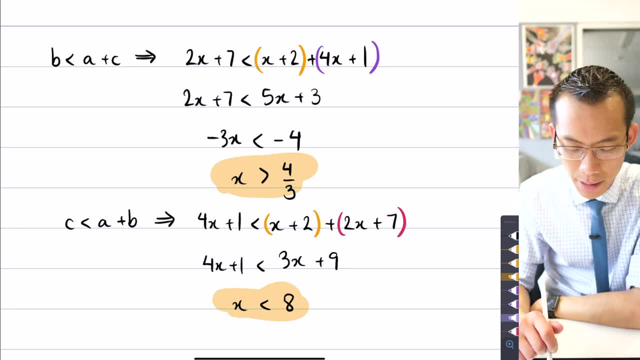 but I can't be seven point nine, nine, nine, nine, nine, nine, because that's not a whole number. In the same way, X is greater than four thirds. I've already excluded that exact value. but I have to go further. I've got to go to the next whole number, the next integer, So that's.